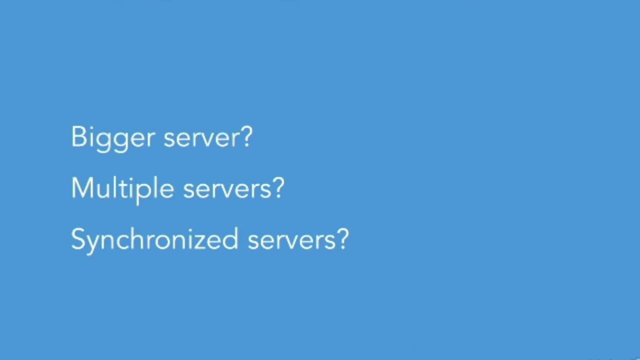 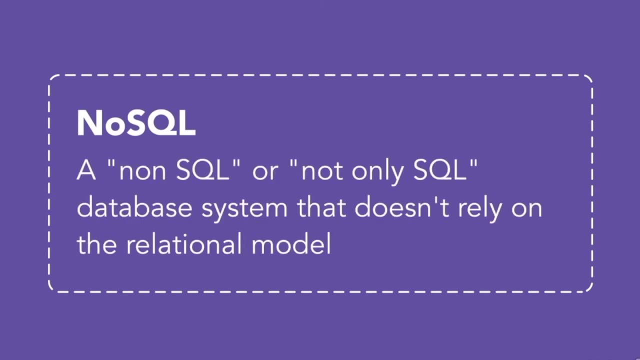 creating relationships. Just dump it in and you're done. That's the idea behind NoSQL. NoSQL was first used as a Twitter hashtag for developers who wanted to move beyond relational databases. It's actually not a slam against SQL. In fact, NoSQL doesn't have very much to do with SQL at all. It's about the 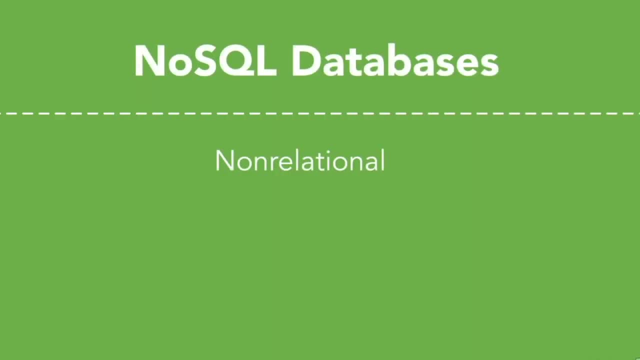 limitations of the relational database model. In general, a NoSQL database should be non-relational, schemaless, clusterless and non-relational. It should be cluster-friendly and, hopefully, open-source. All of these qualities should appeal to a data science team. When a database isn't relational, it's easier to change and 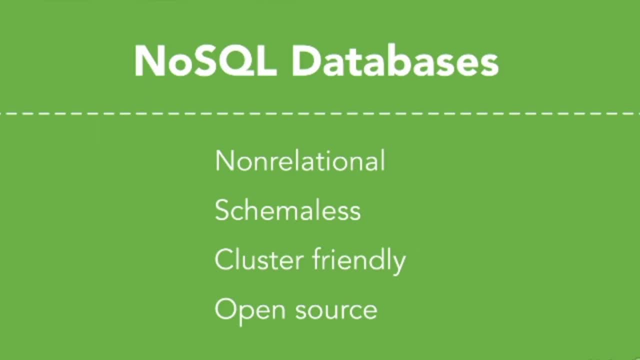 simpler to use. There doesn't have to be a big difference between how your web application works and the way you store data in your database. You won't have to go through the ugly process of creating and splitting tables that already exist to create different views. This is commonly 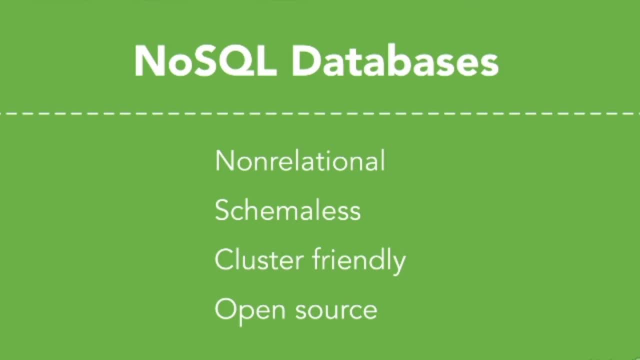 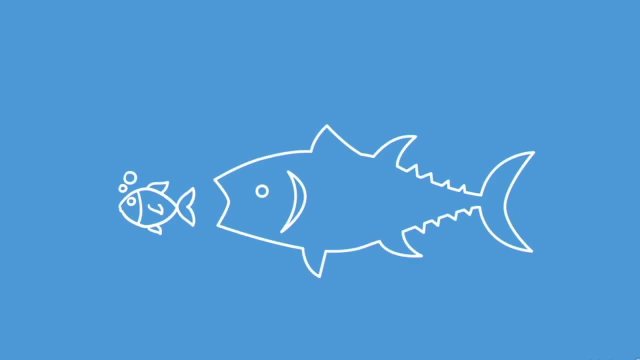 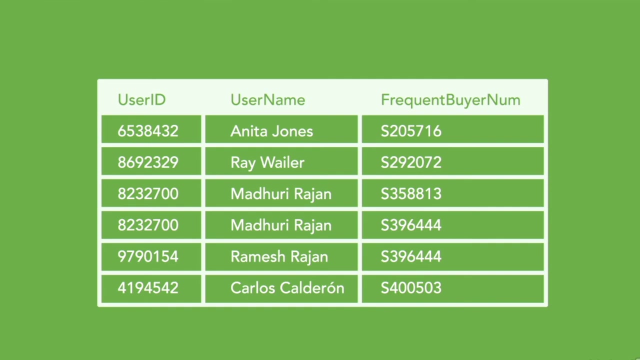 referred to as normalizing your database Without a schema. you don't have to worry about knowing everything up front. Let's say the website was bought by a larger company. This company wants to add your customers to their frequent buyer program With a relational database. this is a serious architectural challenge, Should you have. 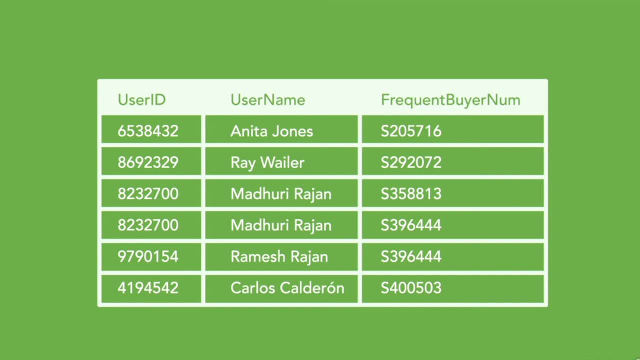 the frequent buyer identified in the customer table. Maybe you need to create a whole new table of frequent buyer numbers. Can a customer have more than one buyer number? Can two customers share the same buyer number? All this needs to be sorted out. You have to rework the database and figure out how to correct for missing data Without 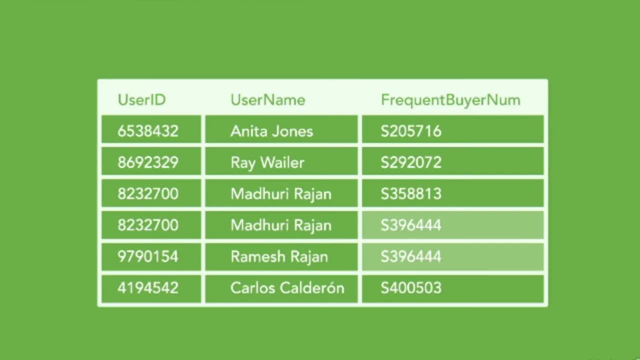 a schema, any new fields become almost trivial. You can just store it as one transaction. If the customer has a frequent buyer number, then it's loaded as part of the transaction. If they don't, then the field doesn't exist. Finally, a NoSQL database should be cluster-friendly. 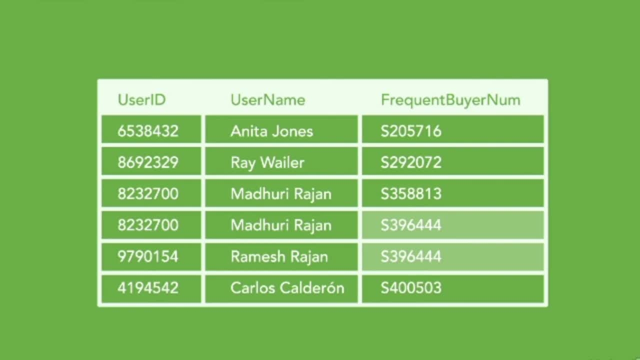 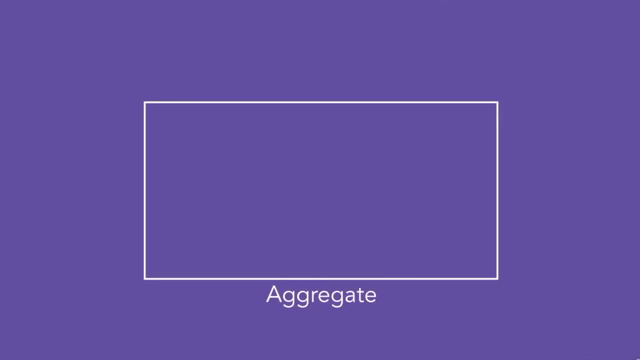 You should be able to store the data in several hundred or even thousand database servers. In a NoSQL database, the record saved in a transaction is called an aggregate. These aggregates hold all of the data They have: the Shoe, the customer address and shipping.